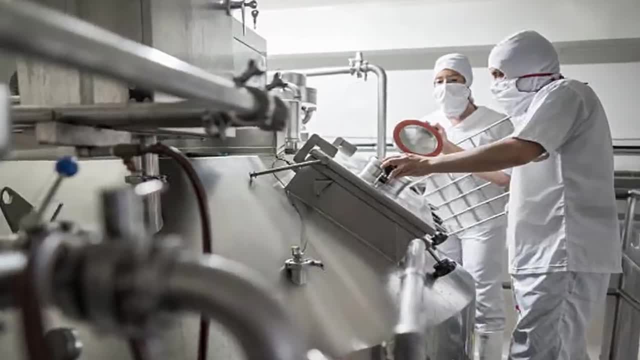 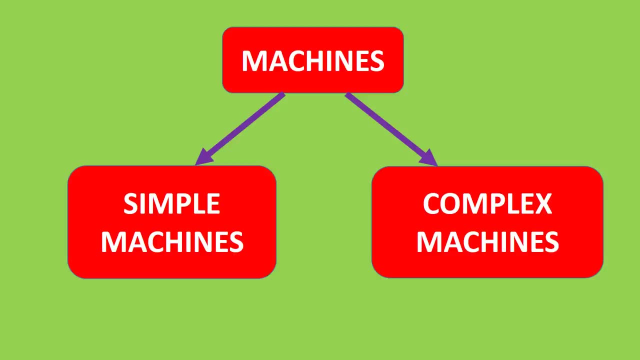 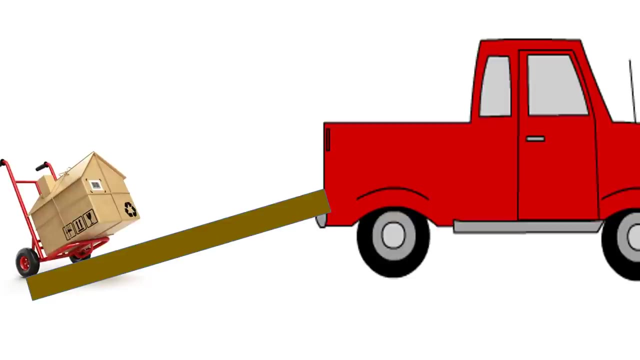 power and time. we need to get one thing done by magnifying our input force. Machines are of two types: Simple machines and complex machines. Simple machines are basic mechanical devices for applying a force and doing work. It helps us to do any work. 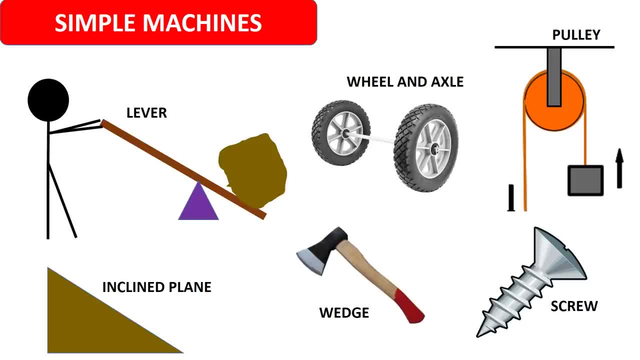 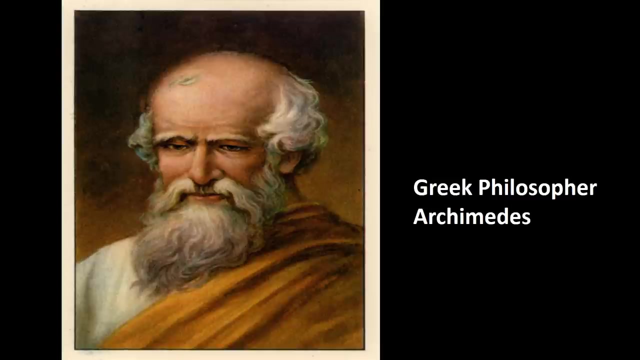 with less effort. There are six basic types of simple machines. They are lever, wheel and axle, pulley, inclined plane, wedge and screw. Simple machines were first discovered and described by Greek philosopher Archimedes: Lever: The lever is made up of a straight, rigid. 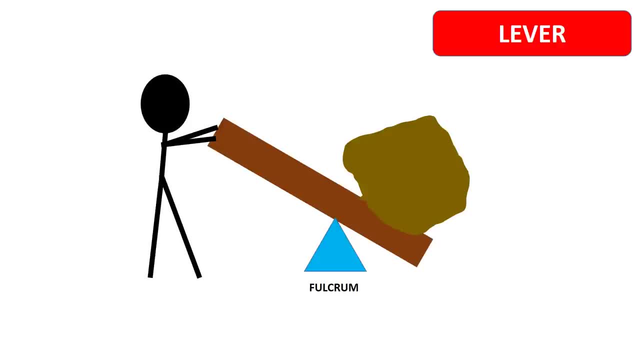 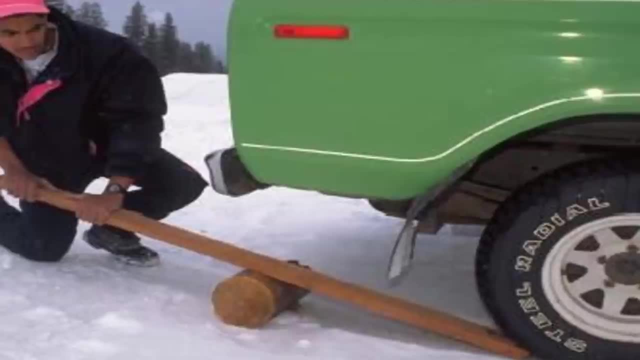 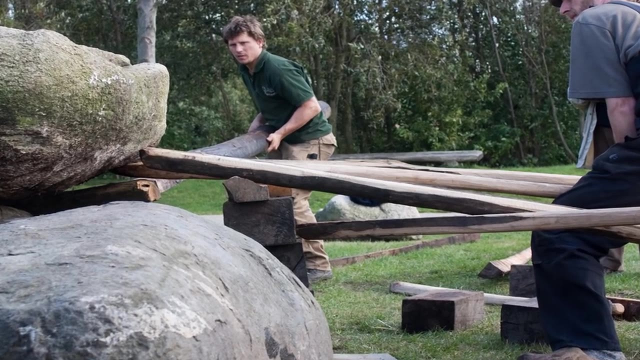 object like a board or a bar, which pivots on a turning point called a fulcrum. Levers make work easier by using leverage, which multiplies the force. When you use a lever, you move a smaller force a longer distance in order to lift a load. a short distance. Parts of a lever. 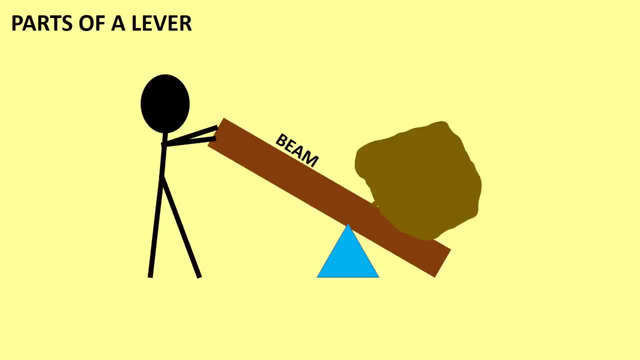 Beam, The physical lever itself, made of materials such as wood, metal or plastic, which can pivot or move on the fulcrum. Effort: The force that is exerted by a person or machine on a lever. Fulcrum: The point at which a lever pivots or hinges. 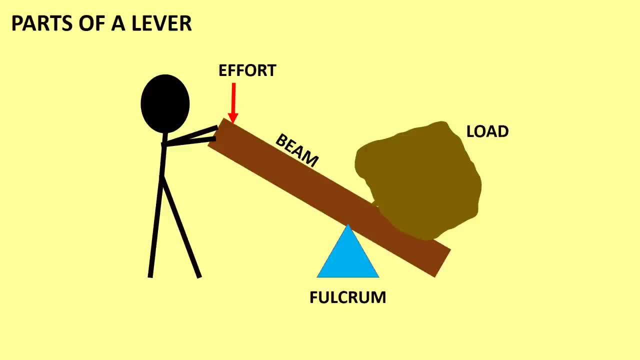 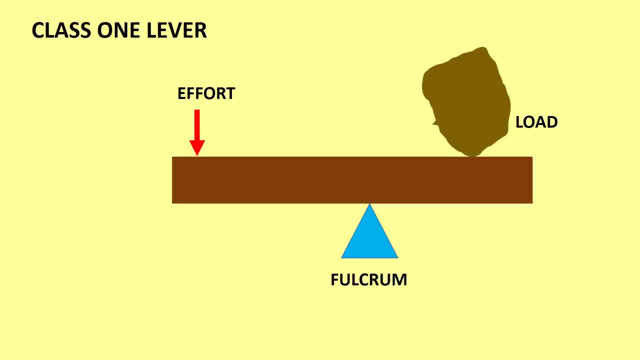 Load The object that is acted on by the lever. There are three lever classes: Class one: lever. In this class the fulcrum is between the effort and the load. The mechanical advantage is more if the load is closer to the fulcrum. 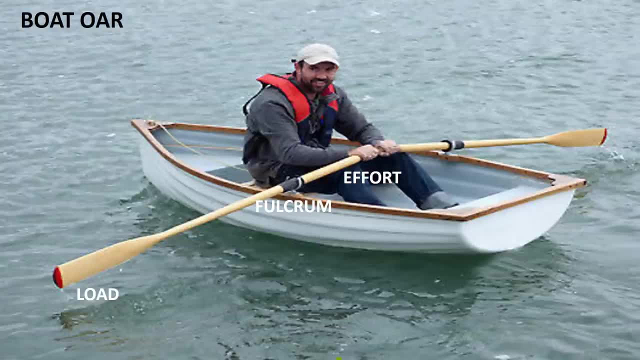 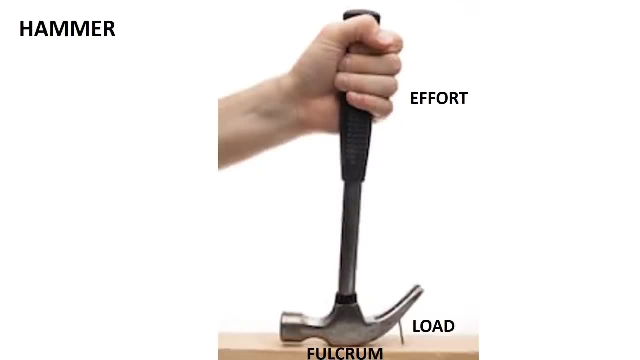 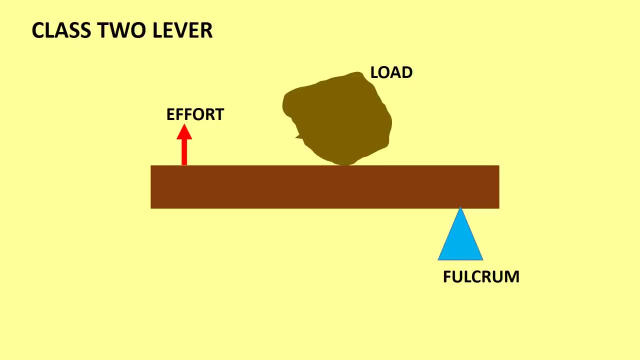 Examples of class one levers are: seesaw oars, boat oars, scissors, hammer pliers, Class 2 lever. In this class the load is between the effort and the fulcrum. The mechanical advantage is more if the load is closer to the fulcrum. 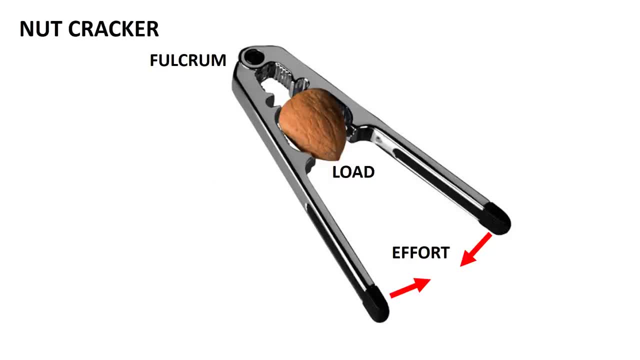 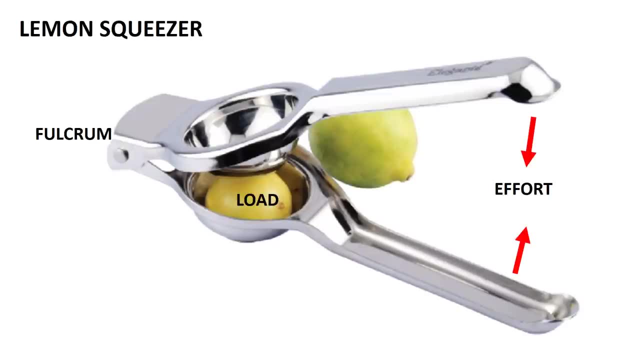 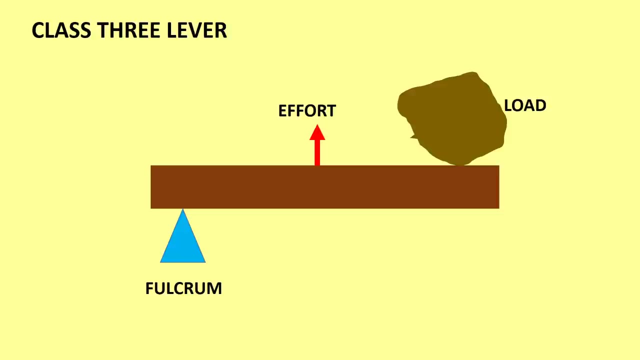 Examples of class 2 levers are wheelbarrows, nutcracker and lemon squeezer Class 3 lever. In this class the effort is between the load and the fulcrum. The mechanical advantage is more if the effort is closer to the load. 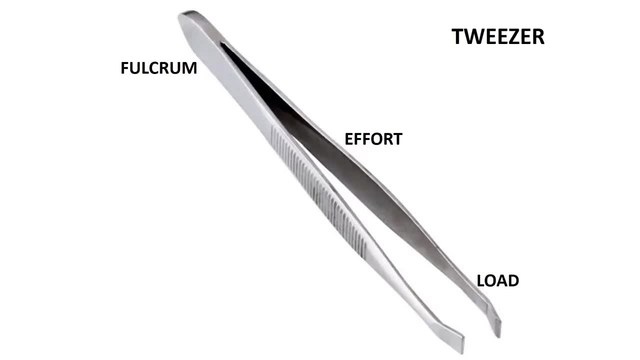 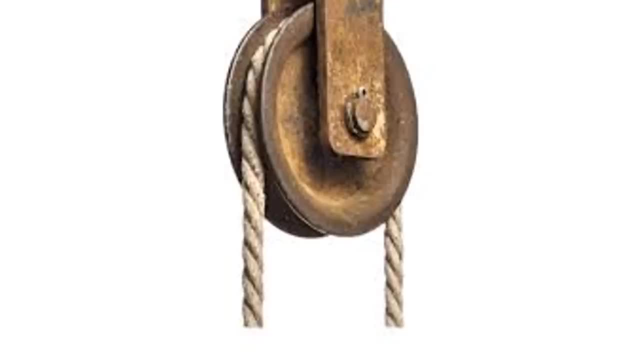 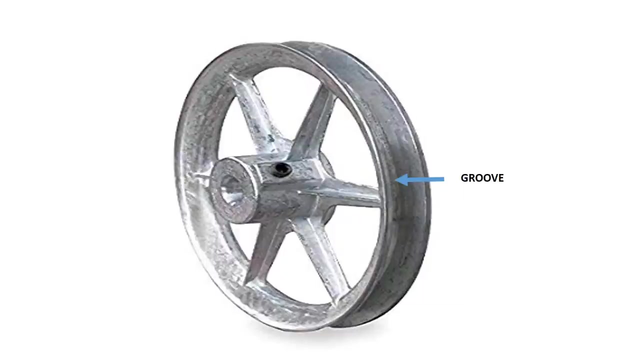 An example of class 3 lever is a guard and shovel tweezers and a rope. Class 4 lever Pulley. A pulley is simply a wheel with a groove in it and a rope in the groove. The groove is important because it helps to keep the rope in place. 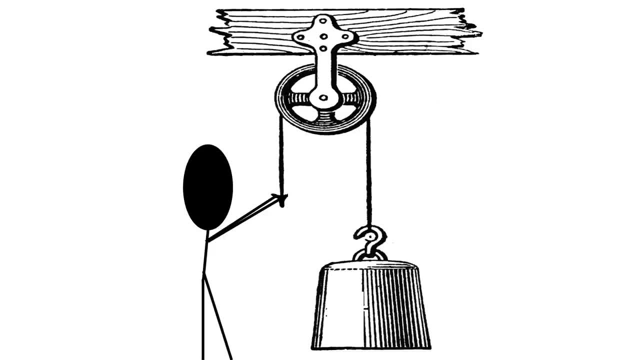 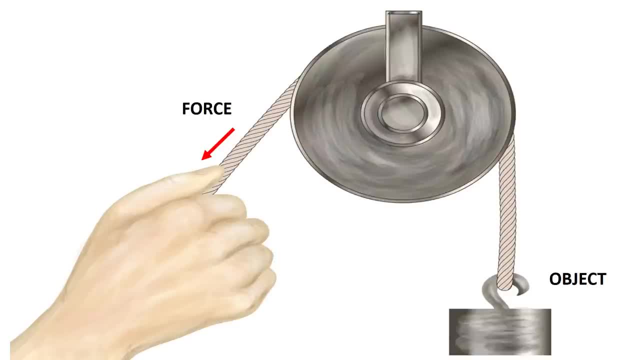 Pulley is used to lift up or lower heavy objects. With a pulley, an object to be lifted can be tied to one end of the rope and a force is applied to the other end by pulling the rope downwards. The downward force. 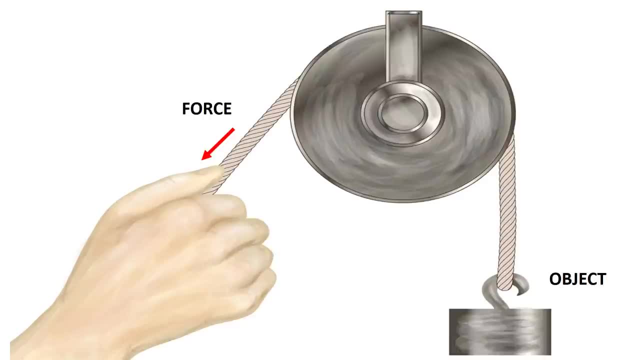 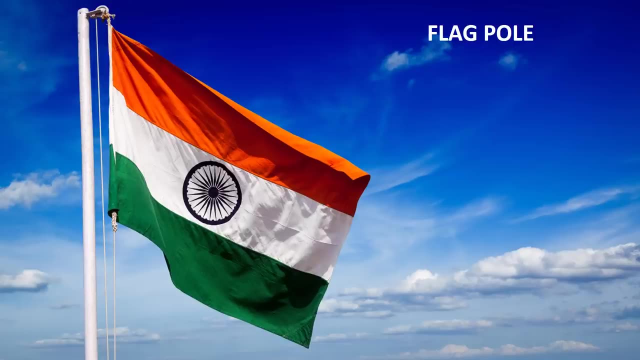 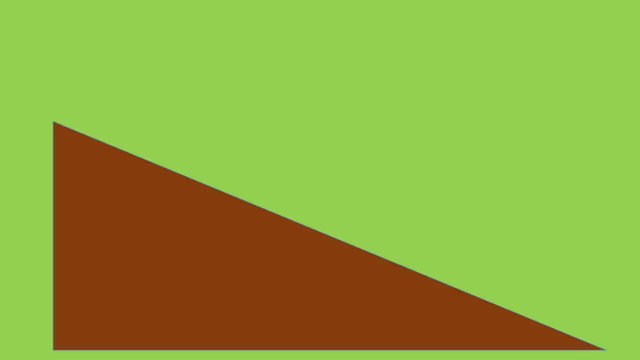 turns the wheel with the rope and pulls the load upwards. at the other end, Pulleys are used in curtains, water, well crate and in flagpole Inclined plane. An inclined plane is simply an even sloping surface with no moving parts. 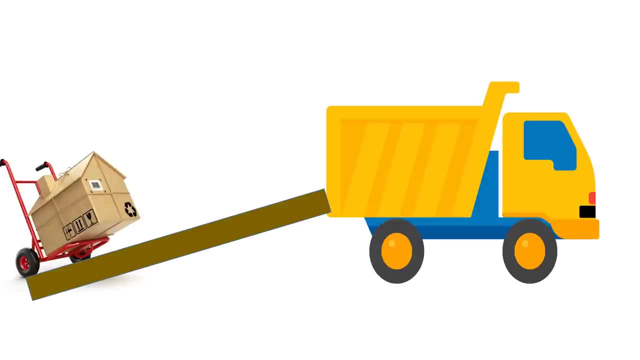 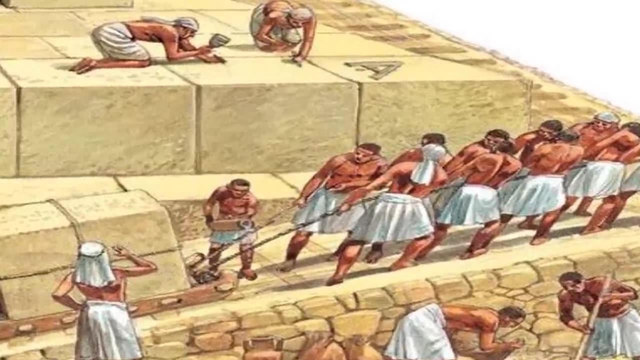 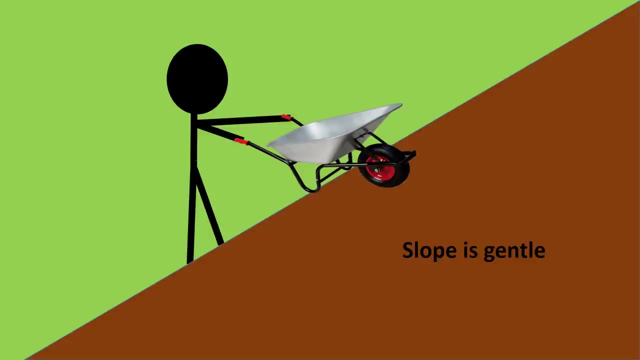 It makes it easier for us to move objects to higher or lower surfaces than if we lifted the objects directly upwards. It is believed that ancient Egyptians used inclined planes to carry heavy stones to build pyramids. If the slope is gentle, a person has to push or pull the object over a longer distance. 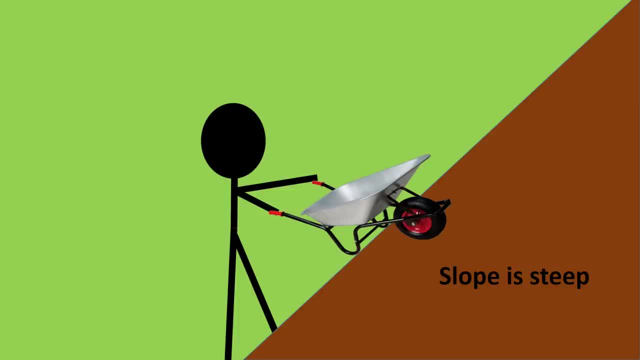 but with very little effort. If the slope is steep, a person has to push or pull the object over a very short distance, but with more effort. Examples of inclined planes are slides and ladders. The inclined planes are sliders and ladders. 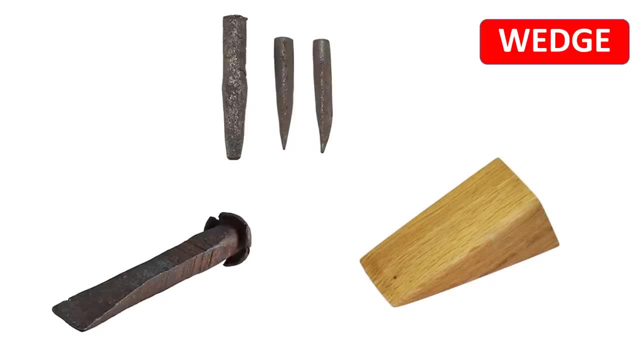 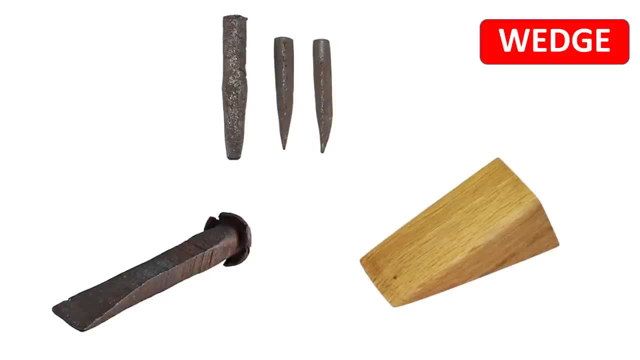 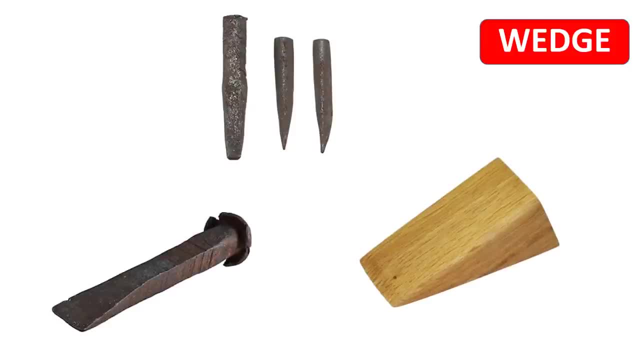 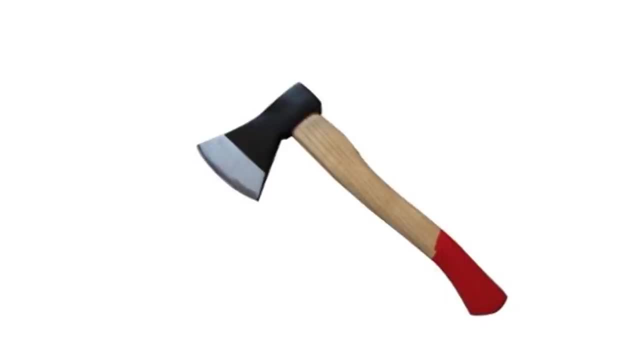 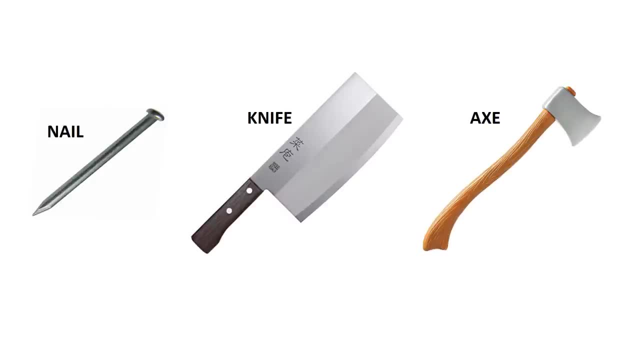 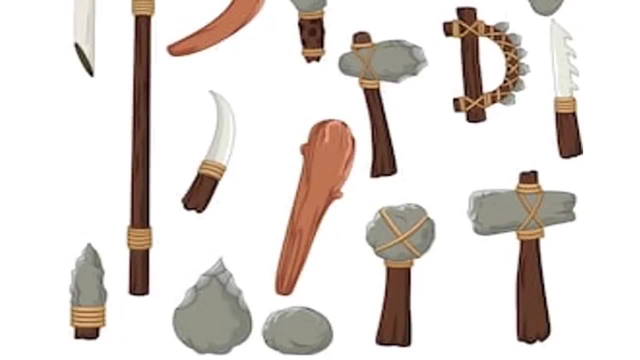 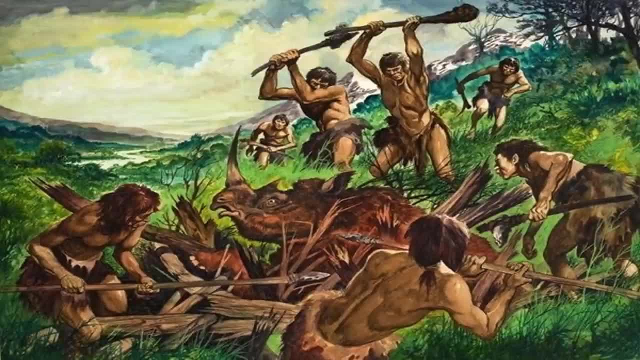 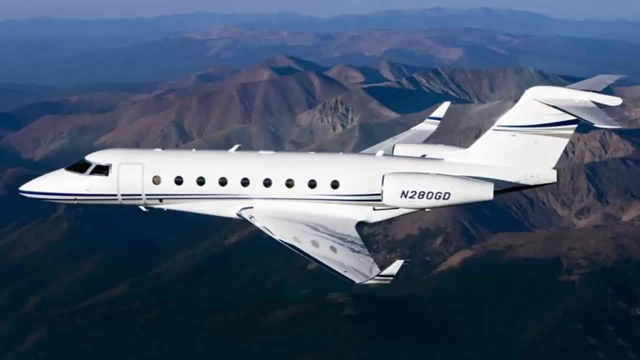 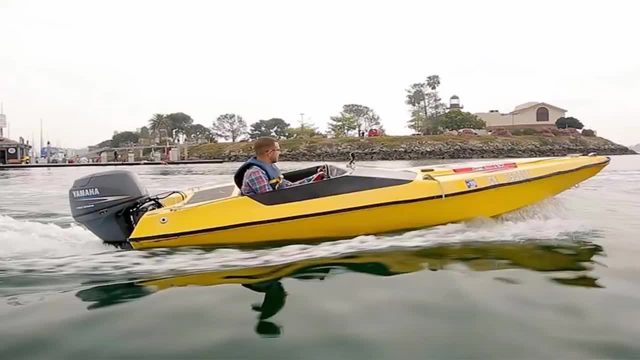 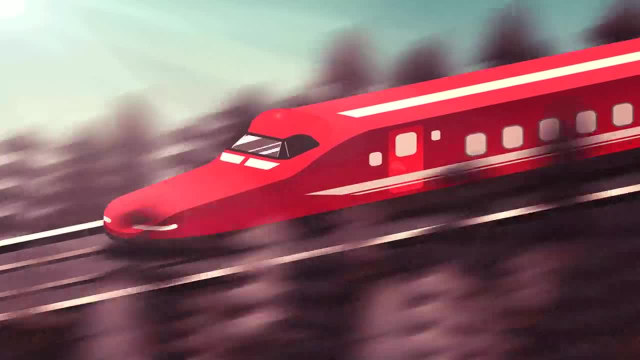 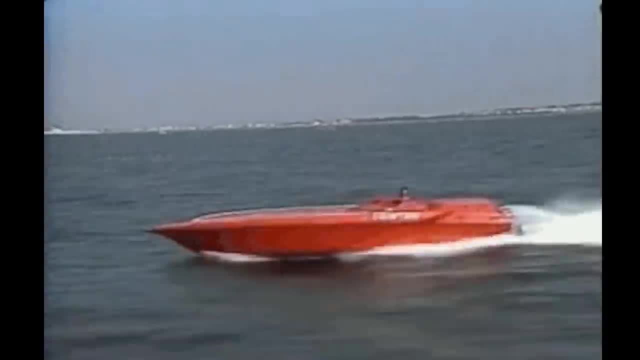 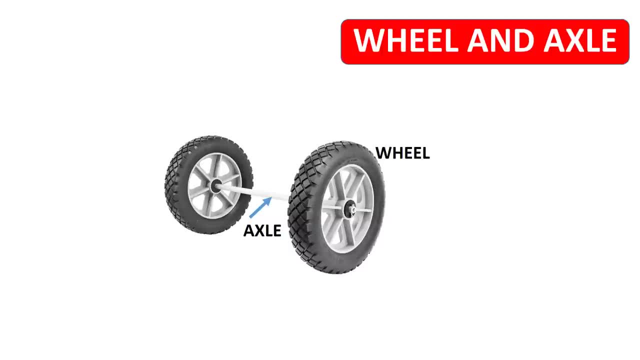 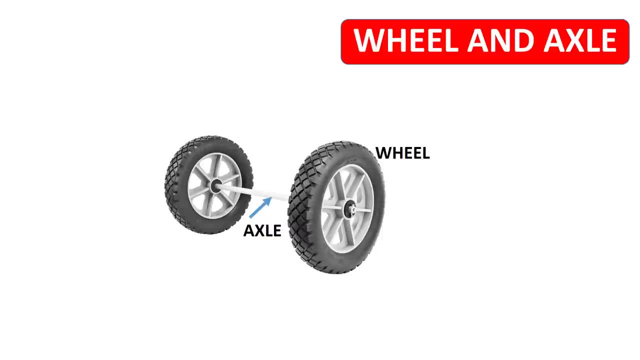 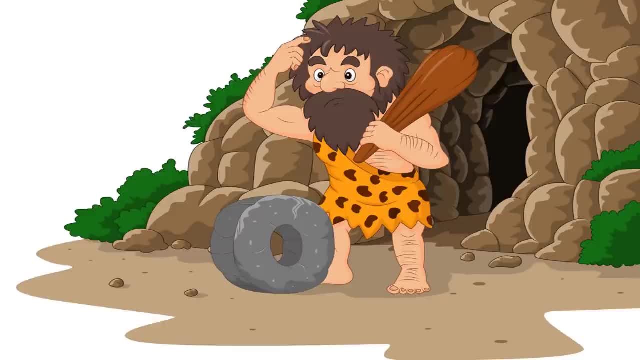 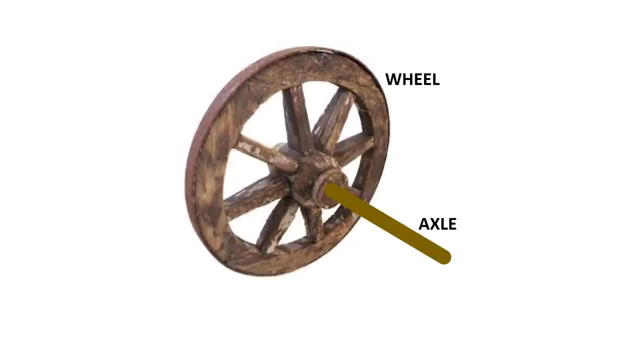 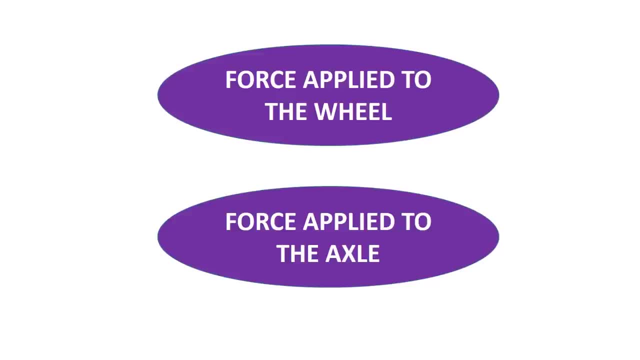 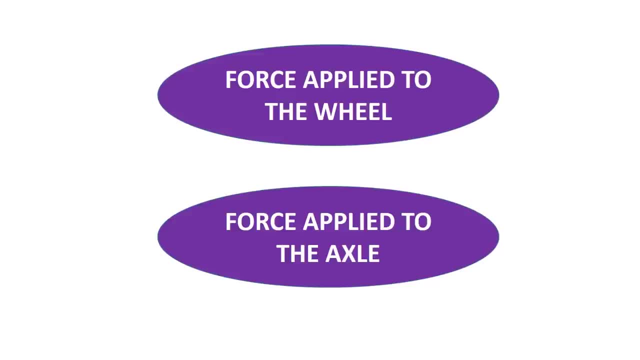 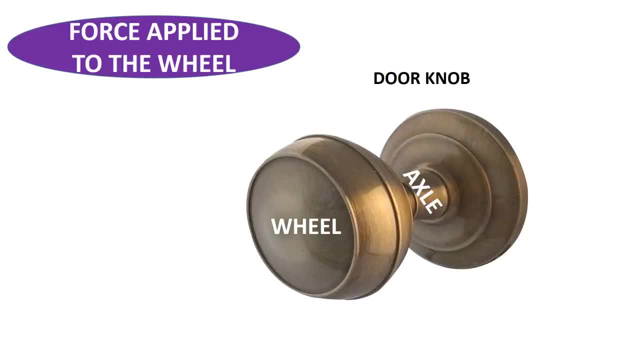 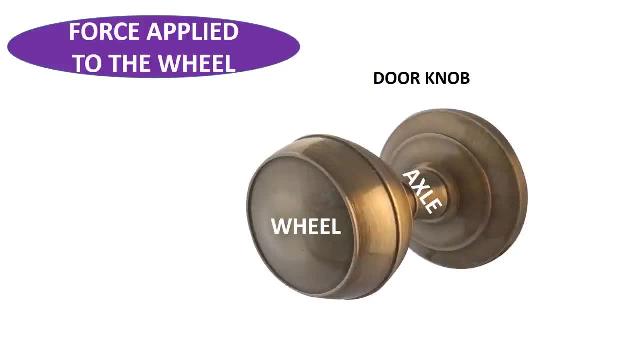 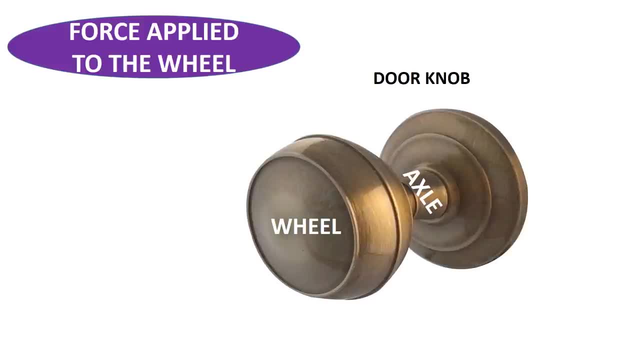 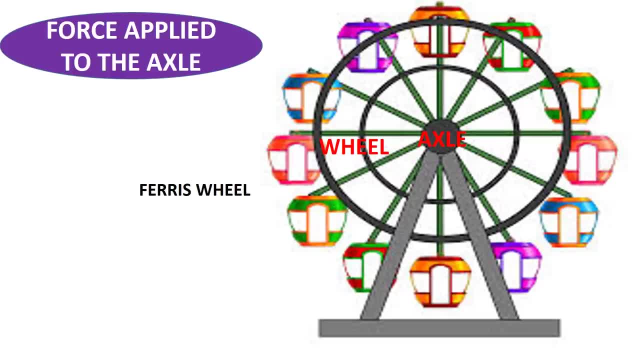 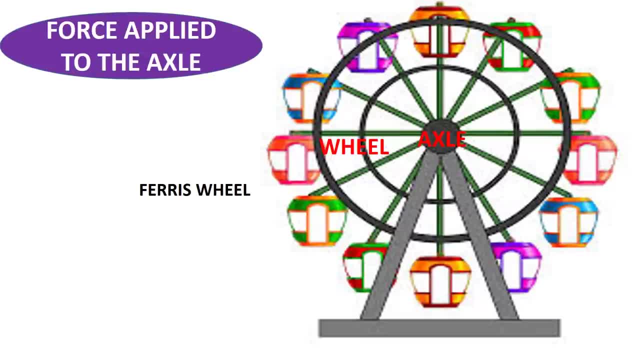 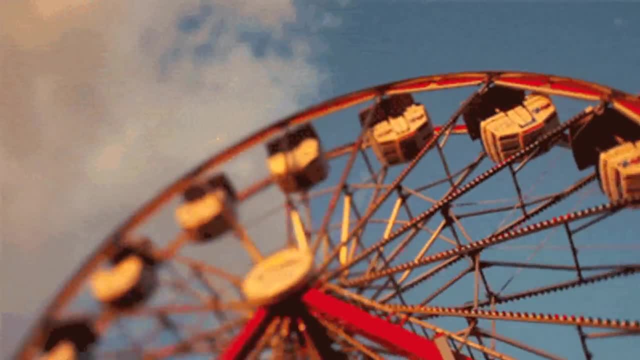 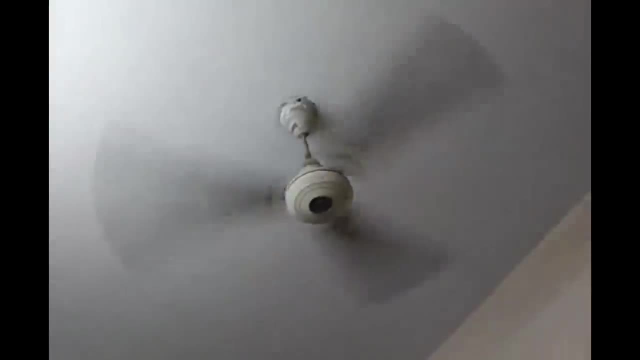 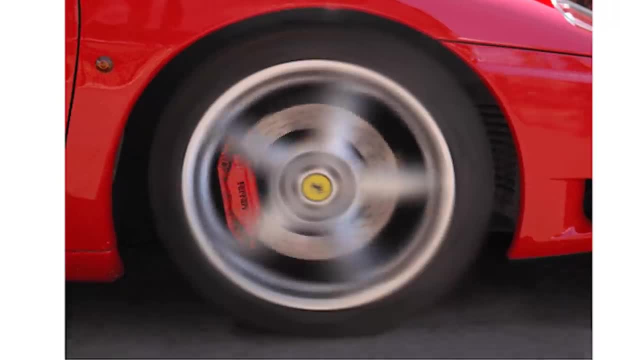 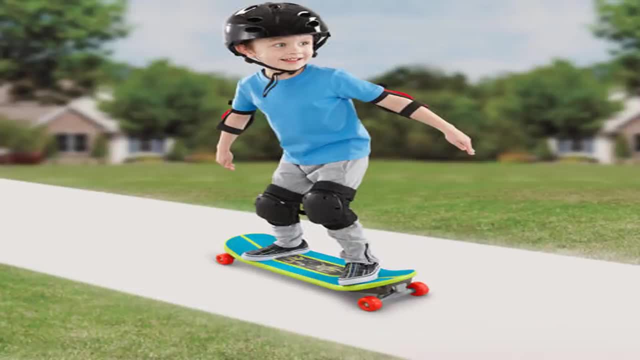 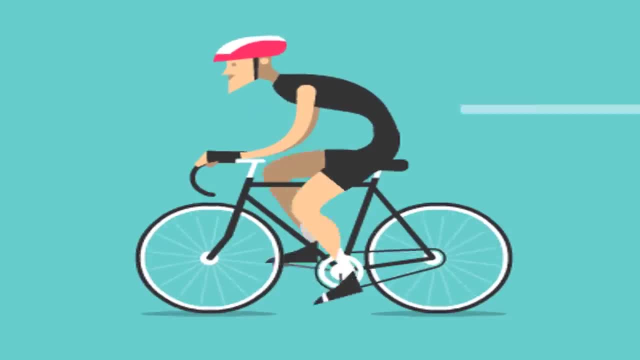 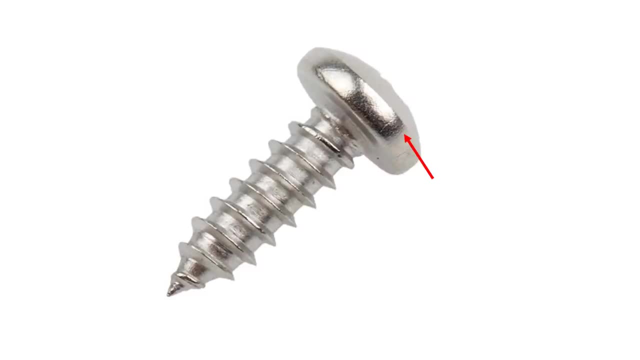 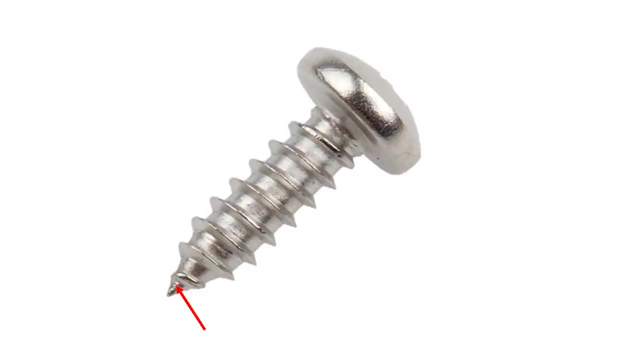 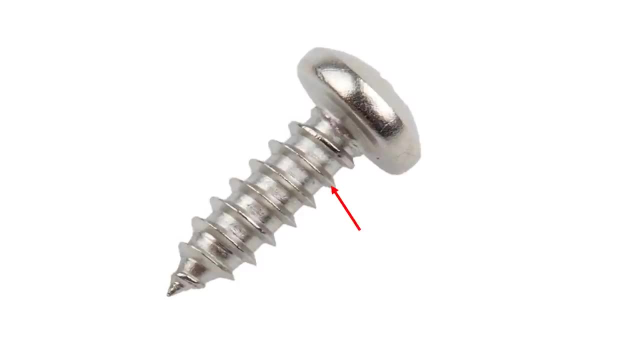 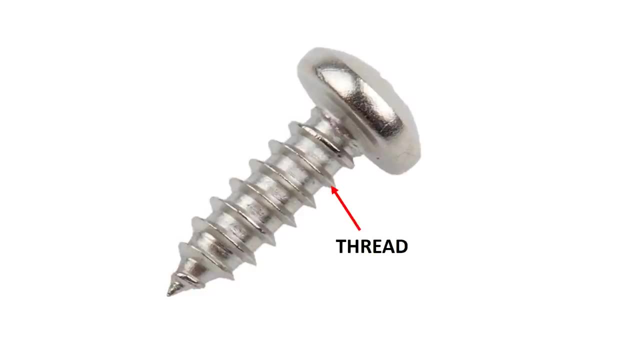 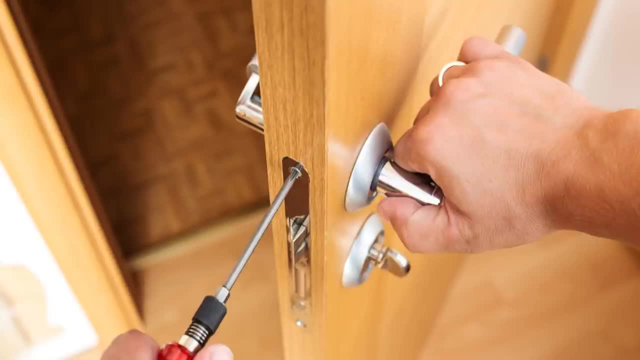 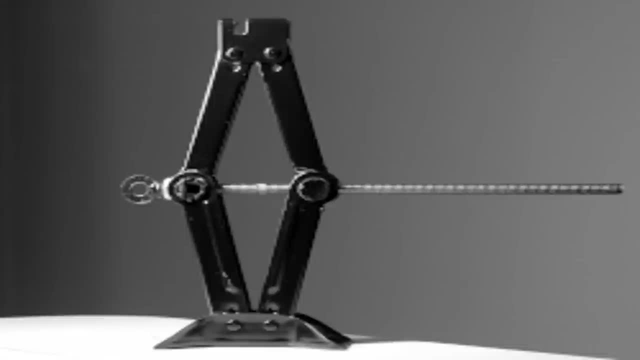 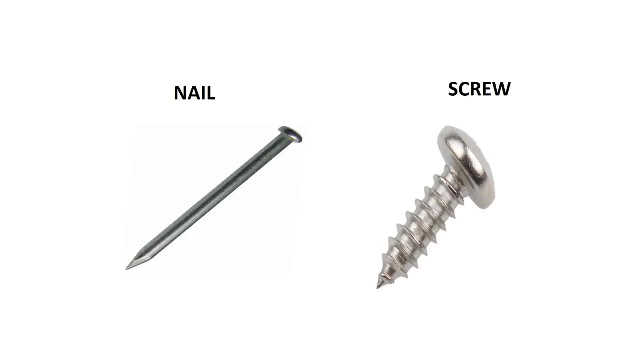 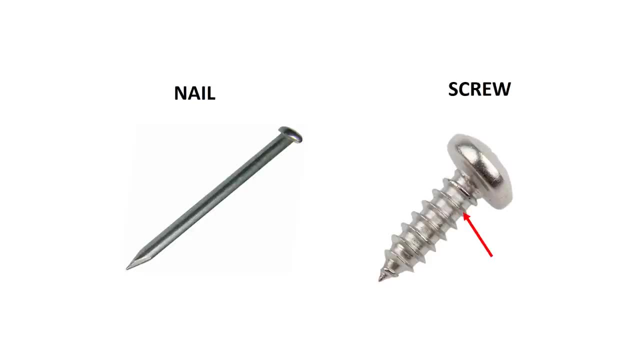 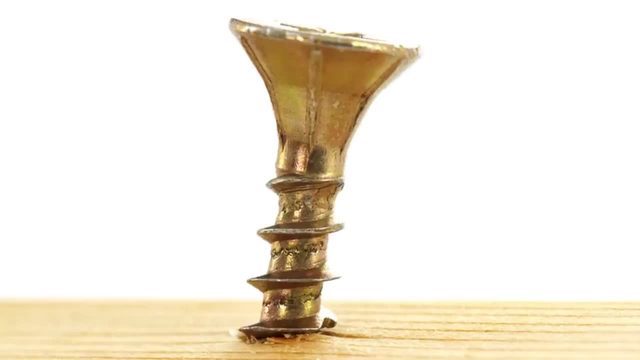 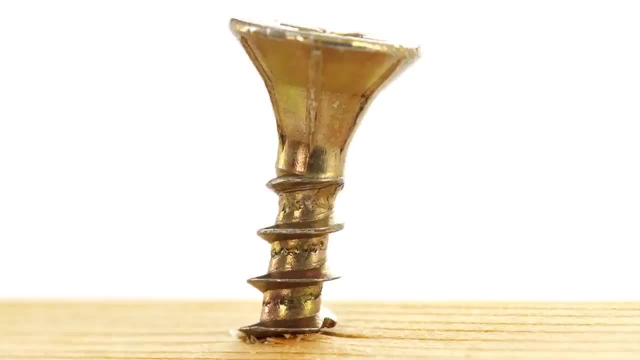 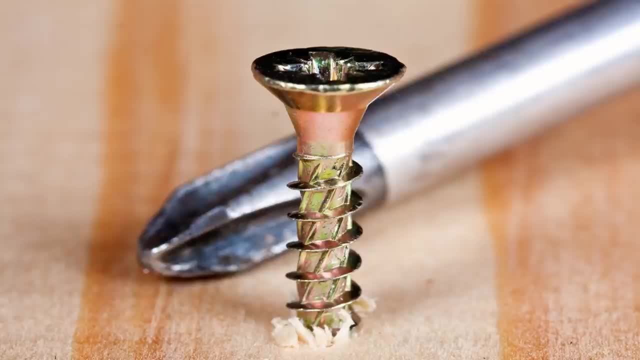 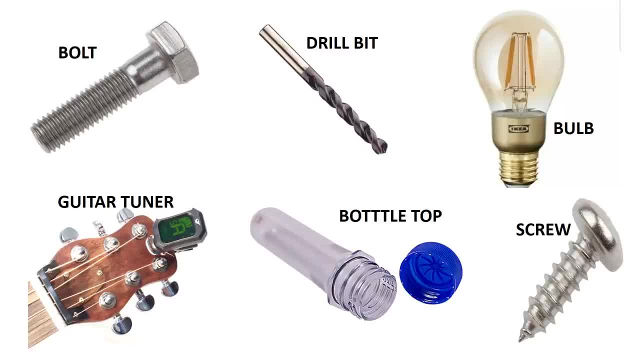